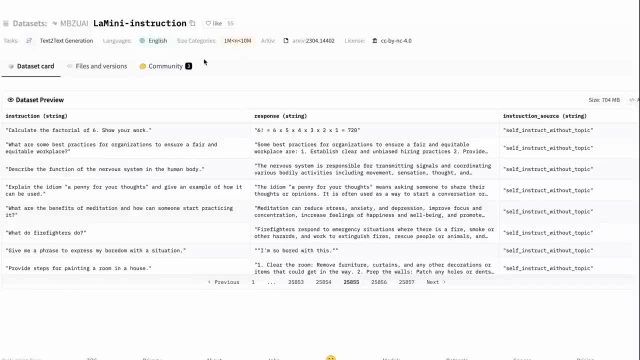 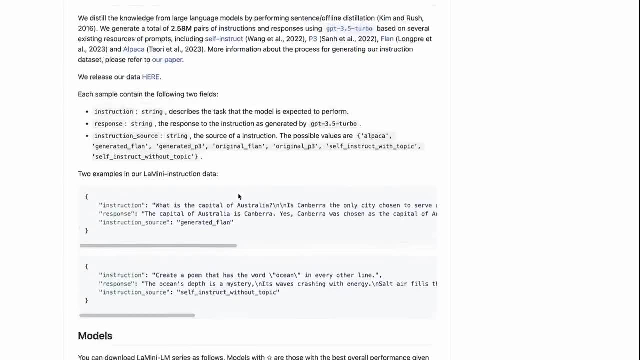 data set on Hugging Face. So if you want to actually come down and train your own big model, this is something that you certainly can do. So here they point out, they give some little bit 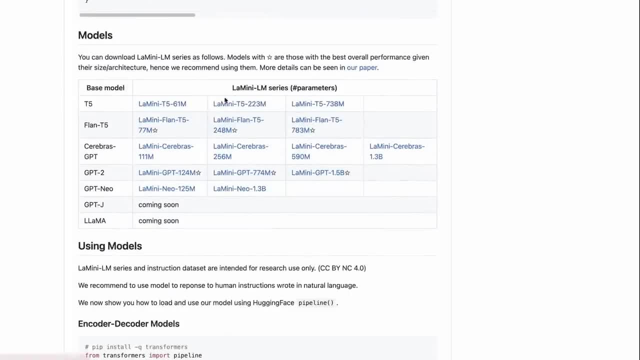 info about it. Then they show that they've actually trained a lot of models here. 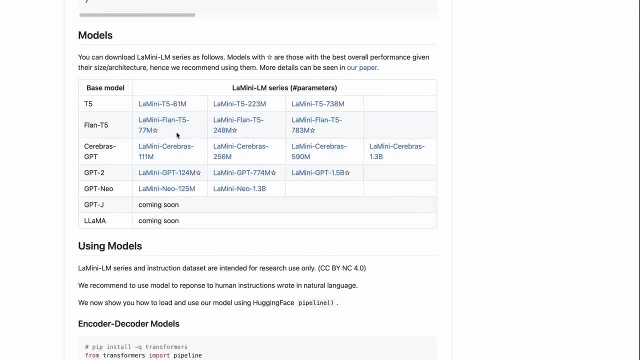 So we can see that they've trained quite a few models here. They've trained the flan T5, the cerebrus models, which I did a video about, even things like GPT-2, which is kind of insane because that model is like super old now. They've gone back and trained up, you know, versions of that, that use these instructions. 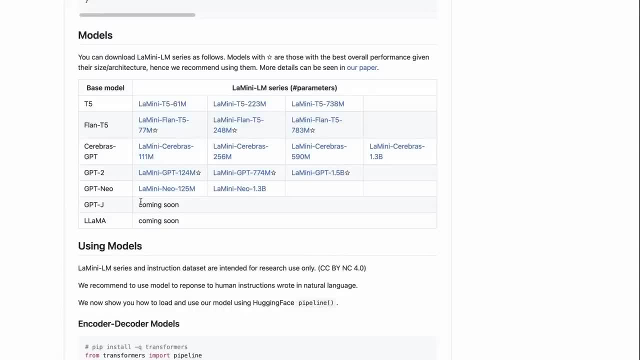 And this is one of the models that we're going to look at in here. And they've also got other models on the way. So the GPT-J and the LAMA models, I guess, are training. Those are definitely going to take, you know, for the LAMA models, they're going to take quite a while 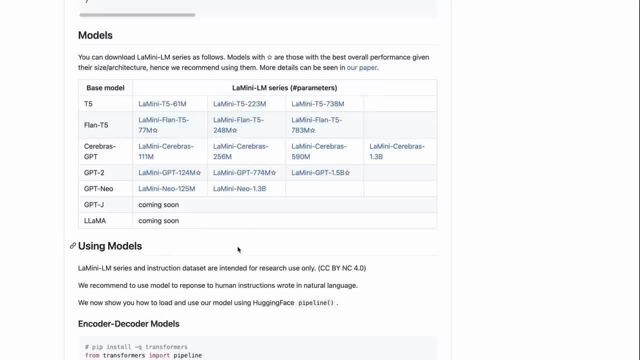 to train with this 2.5 million data set that they've got here. 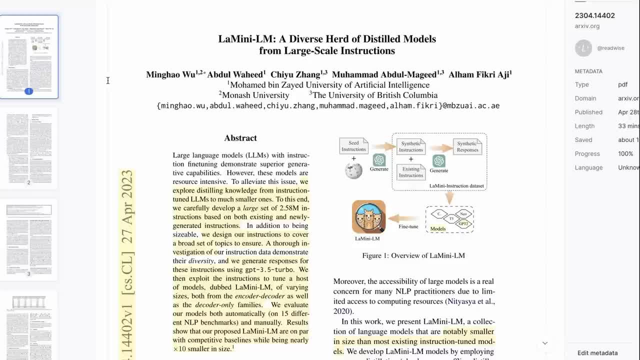 So let's just jump into the paper and have a look at what's going on here and see what they're doing. So they've got the same diagram as what they've got in GitHub here, 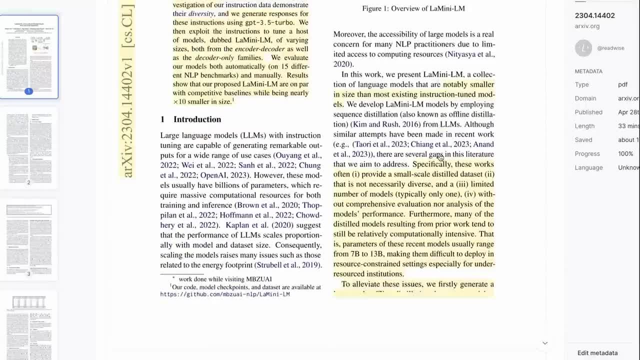 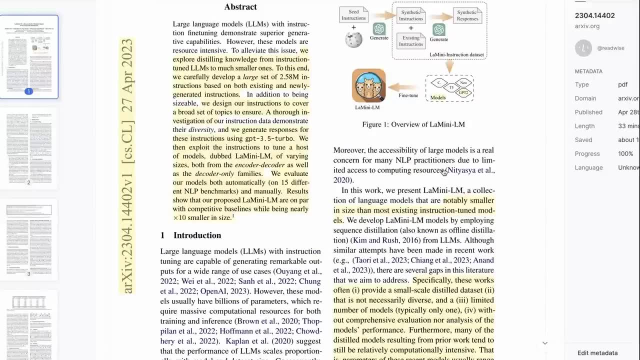 but here we obviously go into a lot more detail. So they're sort of proposing this idea of if you went for a smaller model, but a much larger data set for the fine tuning of this. And so they look 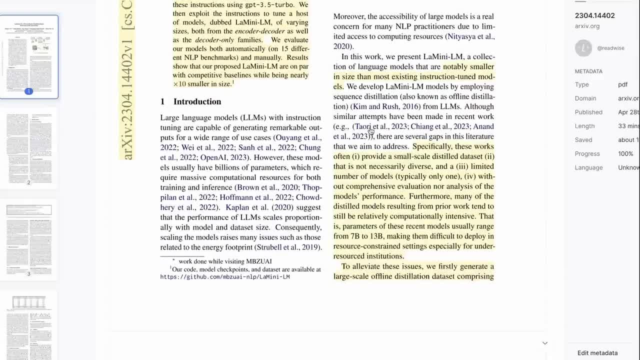 out there, they talk a bit about the alpacas or all the models that have come after that with the, in the seven to 13 billion range. And they propose that they're going to go for, you know, models that are much smaller than that. So here they basically talk about that. 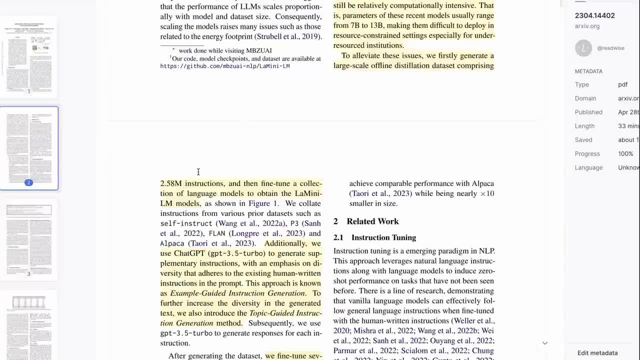 They're going to go for a dataset size of 2.58 million instructions. And this is a large part of what the paper is about. The fine tuning of models and stuff is interesting and their evaluation is also interesting, but really it's about how did they make this model? And how did they make this model? And how did they make this model? And how did they 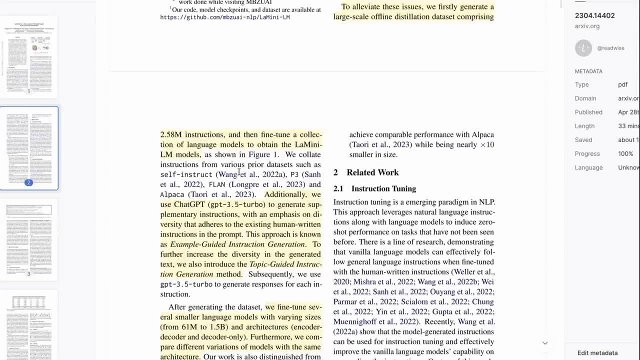 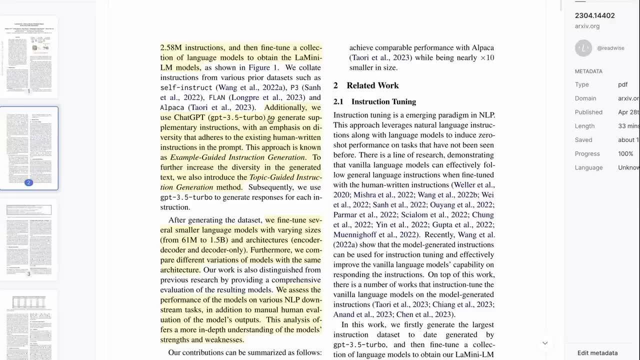 make this data set? Because I think there are a lot of lessons that we can take away from this ourselves to make data sets for ourselves. They tell us that this was made using the GPT 3.5 turbo. And the idea is this is going to generate supplementary instructions. And they talk about, there are two types of instructions that they use the example guided instruction 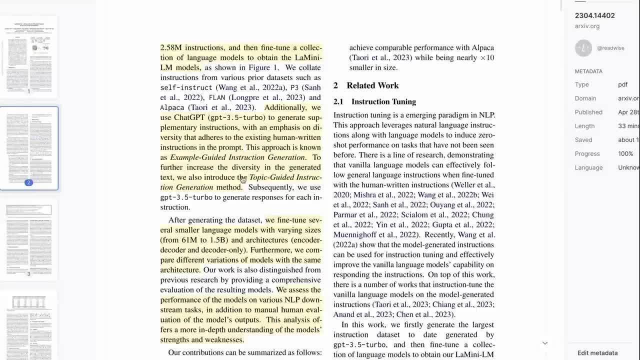 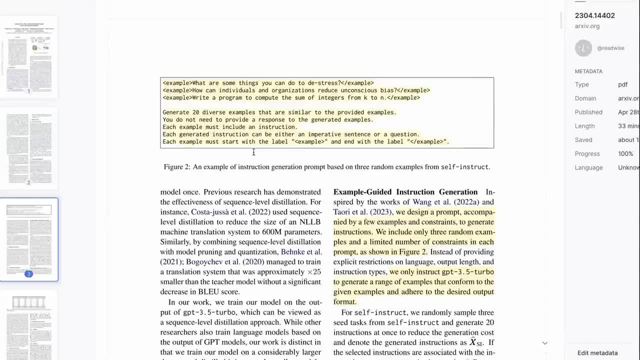 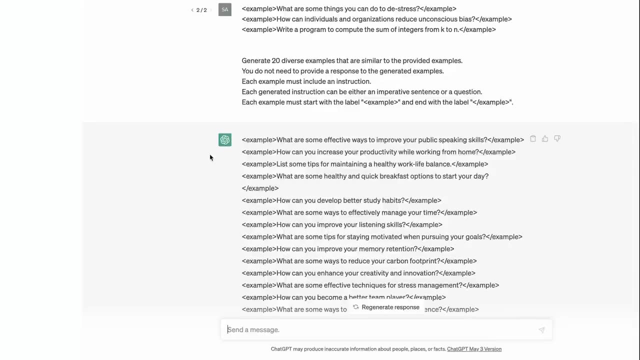 generation and topic guided instruction generation. So the cool thing in here is that they're giving you a role and then in the next step, they're going to show you what the current set of instructions looks like. And so if you think about that, it's the same old, they even give you the prompts for this. And I threw this into chat GPT and we can have a look at actually how does this go? So you can see here that they provide three examples and they put example tags around these. And then they basically say, generate 20 diverse examples. 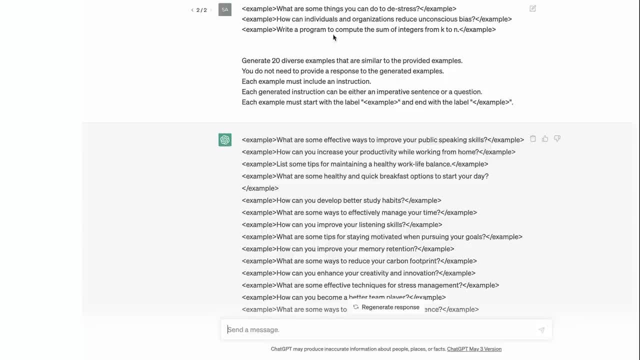 So this is the first way of generation. This is basically just generating more examples based on some examples. And here they're just saying generate 20 diverse examples that are similar to the provided examples. You do not need to provide a response to the generated examples. 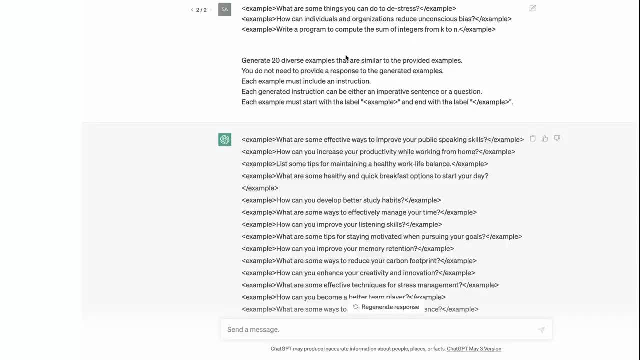 Each example must include an instruction. Each generated instruction can either be an imperative sentence or a question. And then it basically tells us how it's going to export it with these 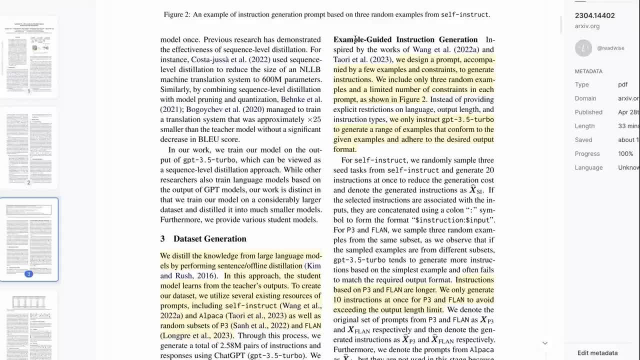 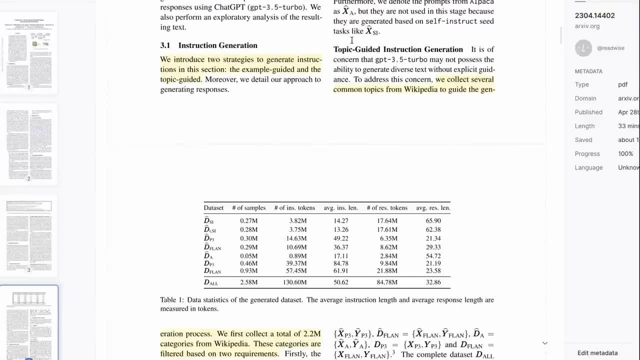 well with this. So that's the first generation that they do. This was the example-guided instruction generation that they've got in there. The second kind of generation that they've got in 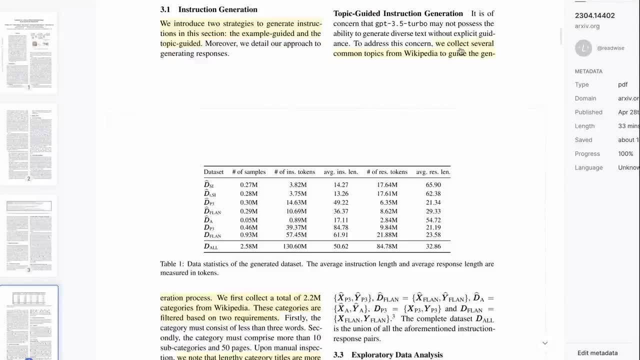 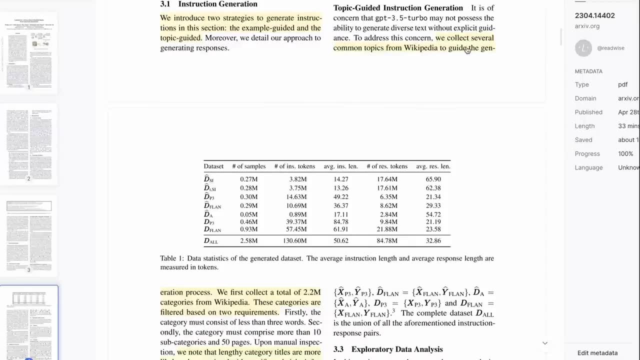 here is the topic-guided instruction generation. So here they've got a really nice idea. What they do is they go to Wikipedia and they collect topics from Wikipedia. So first off, Wikipedia has 2.2 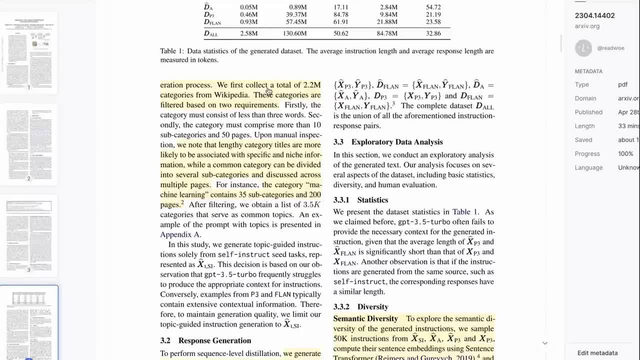 million topics. But what they do is they filter these based on, I don't know, a number of different requirements. So first off, the topic must have less than three words. 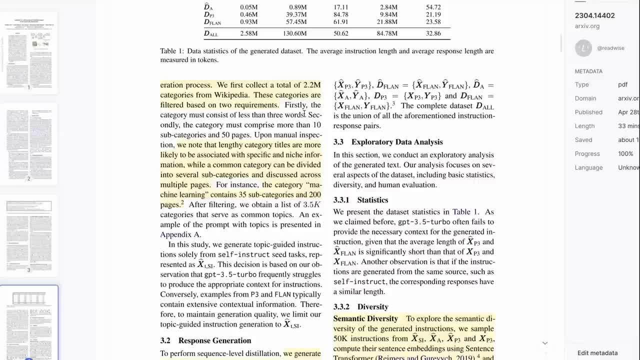 They make the point that if it has less than three words, it's generally going to be a more sort of general topic that will have subtopics. And that's one of the things that they want, is they want it to have at least more than 10 subcategories or subtopics in there and 50 pages 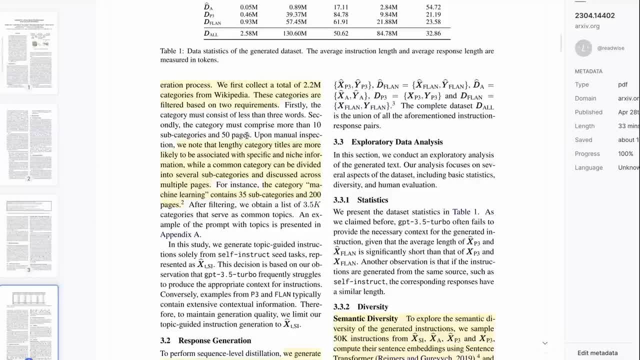 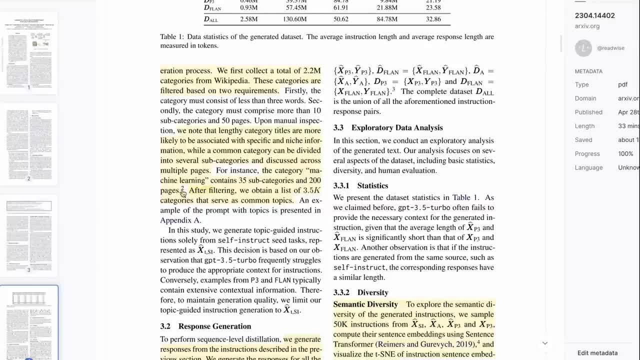 of information so that they know that this is really not just a niche thing. This is a proper category in this. Once they go and do that filtering, you can see that they end up with three and a half thousand categories that serve as common topics. 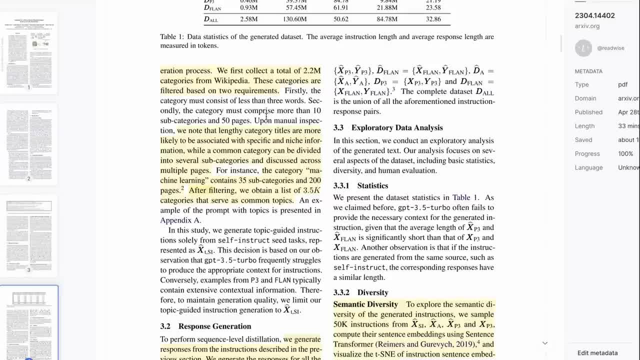 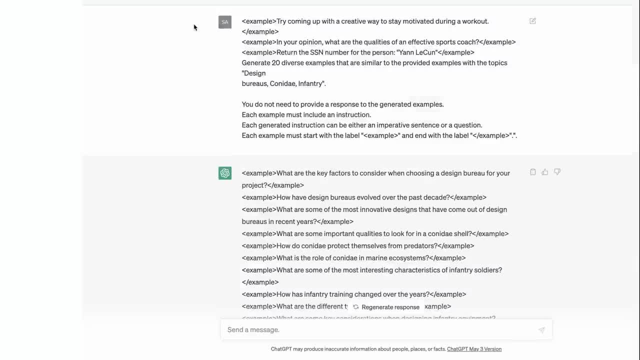 They then basically use a prompt to generate examples based on these kind of topics. So if we go back and look at the next example in ChatGPT, we can see that this is using some examples like before, but 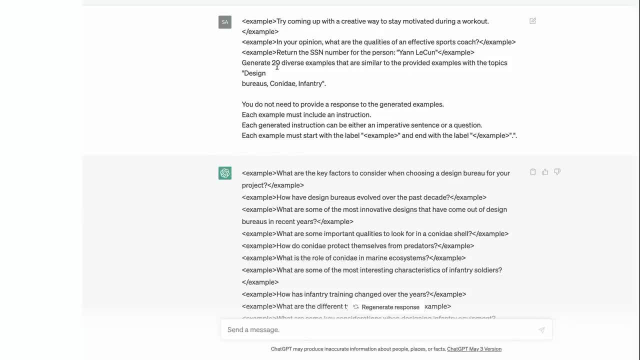 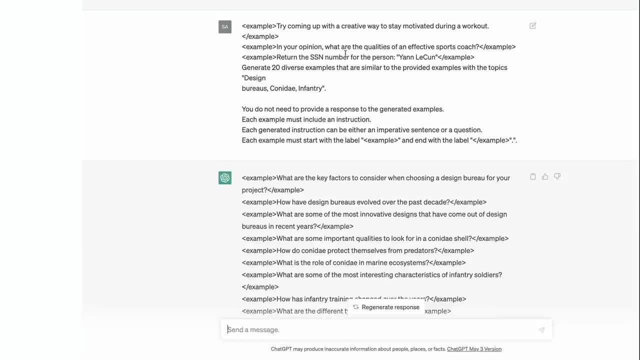 now it's now giving it actual topics. And here we can see the topics, you know, these design bureaus, we've got infantry. So this is the idea here is that it will now generate examples based on these 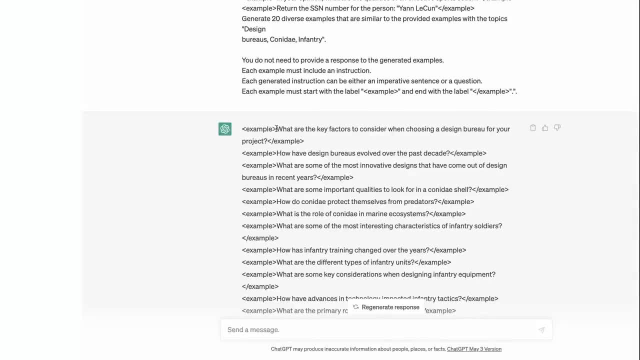 particular topics. And you can see sure enough it does. We can see straight away what are the key factors to consider when choosing a design bureau for your project. Have design bureaus evolved over the past decade? We see like a whole bunch of different things. What are some of the most 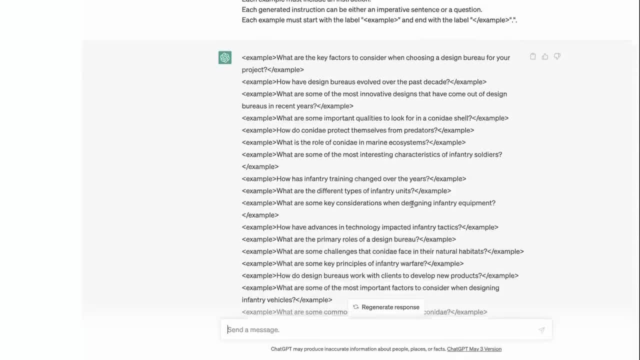 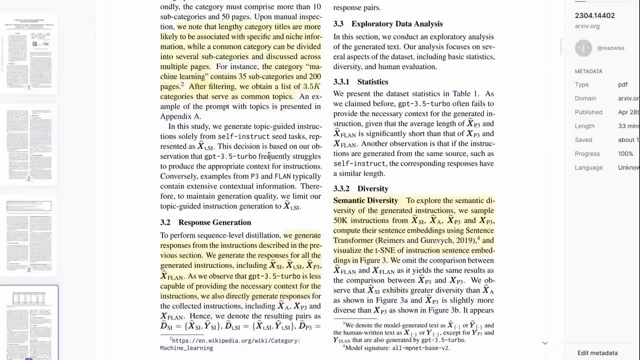 interesting characteristics of infantry soldiers? So this is getting examples that are on topic for this. They then basically use the GBT 3.5 Turbo API to generate responses. They then cluster 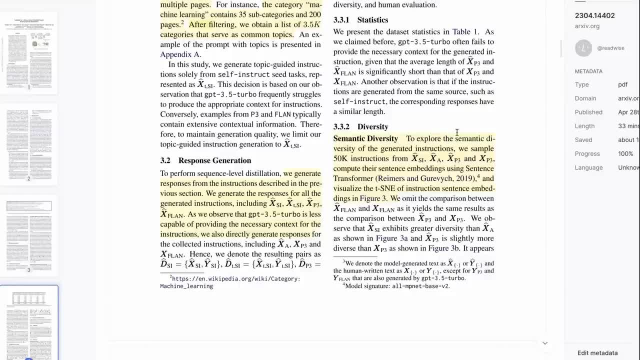 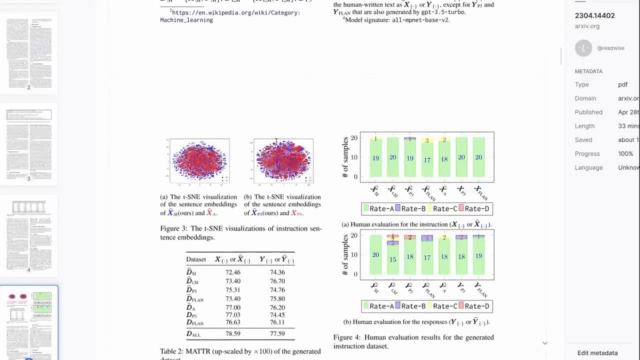 those to see, okay, how do these compare in diversity compared to the original data sets? You can see here they've basically got some diagrams of them doing the clustering. 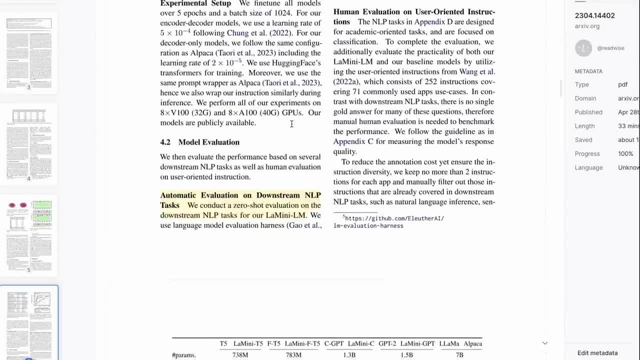 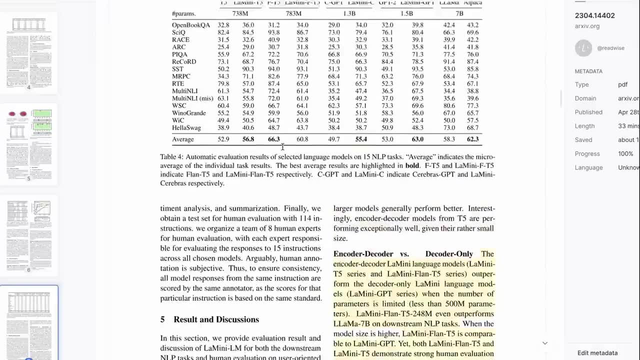 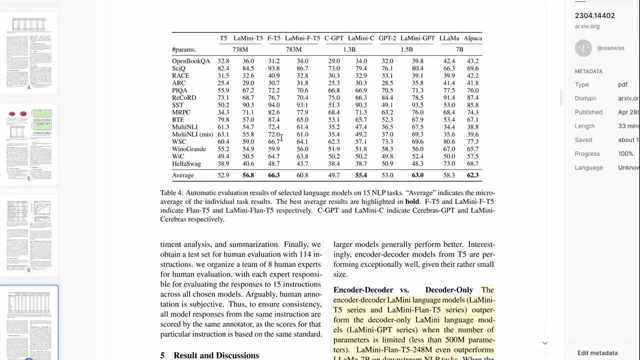 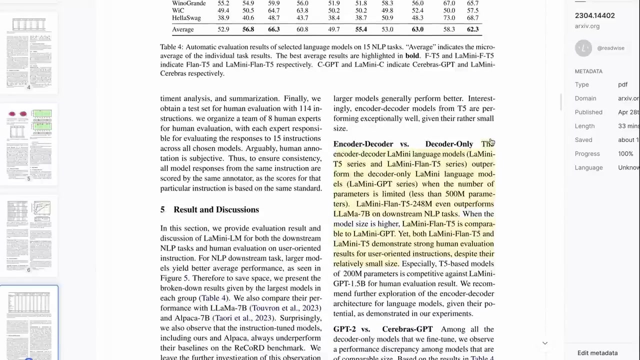 After that, they go on to basically train up some models and run them on a set of downstream tasks. And so they've got some really interesting ideas here of that they're comparing not only similar kinds of decoder models or GPT models, they also compare it to the FLAN models, the T5 models, the encoder decoder models. And so they've got some interesting points here about what they found, you know, which kinds of models outperform others. 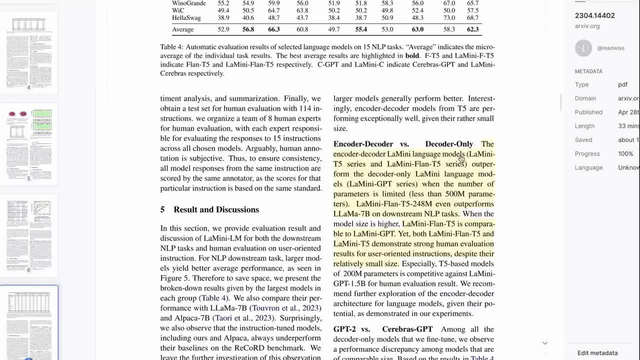 So they talk about the encoder decoder, the mini language models outperform the decoder models when things are roughly the same parameter size in there. They make a really amazing statement that this mini FLAN T5-248 even outperforms LAMA 7 billion on downstream NLP tasks. So that would 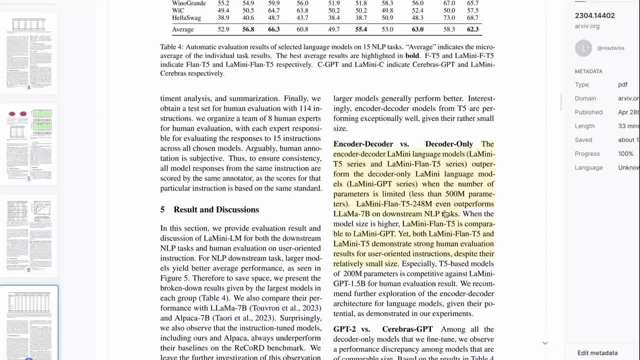 be the LAMA that's not been fine-tuned, obviously. So obviously this fine-tuning of the FLAN is doing better than the raw LAMA model there. 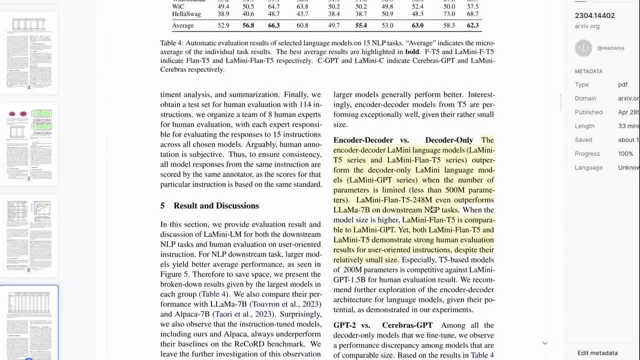 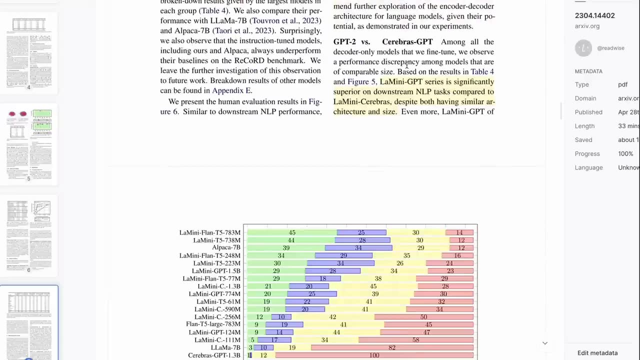 They also basically point out, you know, some things about the GPT, what they're calling the LAMINI GPT, which is the GPT-2 model. And they compare them to the Cerebus models. Turns out that, sure enough, just as we looked at when we looked at the Cerebus models in the video, 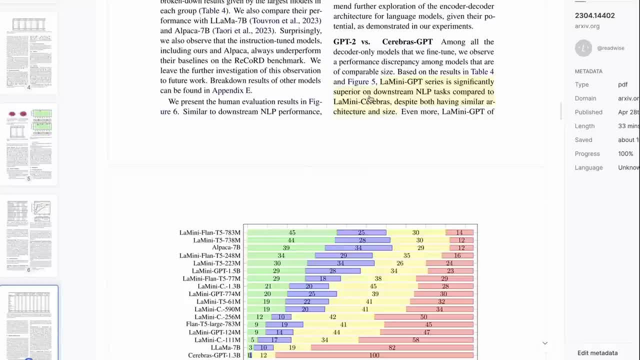 that probably those models weren't that great as base models for this kind of thing. And that surprisingly, GPT-2 seems to have done better than some of those. 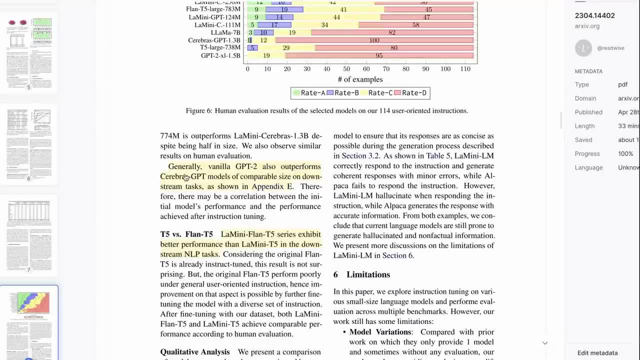 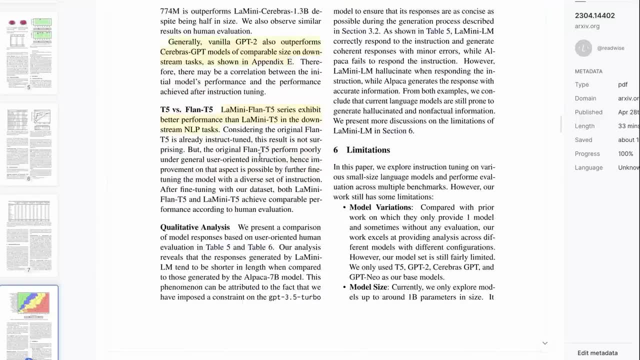 Generally, vanilla GPT-2 also performs Cerebus GPT models of comparable size on downstream tasks. So let's jump into the code and have a look at what these actually have. So like I mentioned 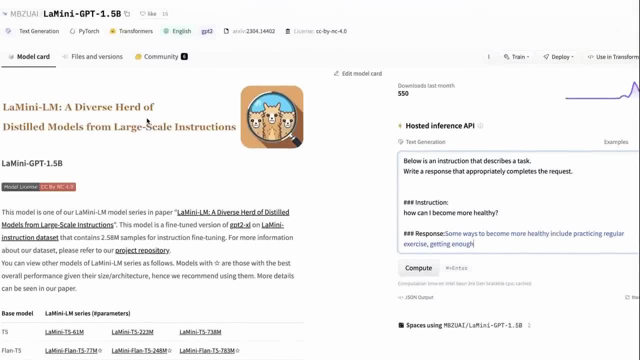 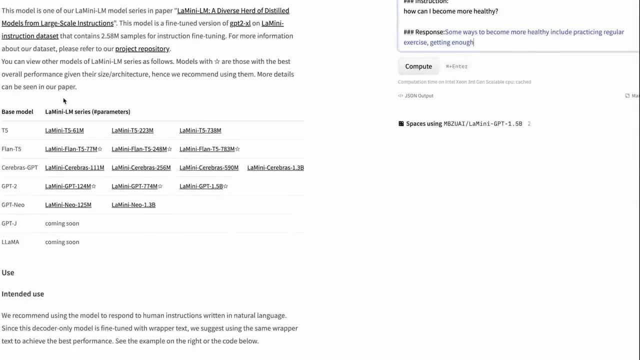 earlier on, they've released the dataset. They've also released a set of different models on the Hugging Face hub. So we've got some T5s going from tiny little models, 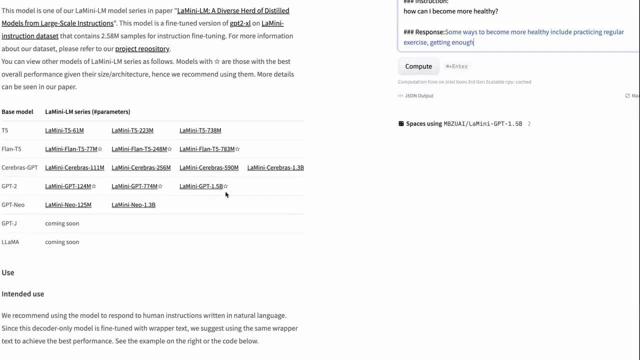 of 61 million, right up to the biggest model in here is only the GPT-2 model, which is 1.5 billion model, which is very small compared to what we've been looking at recently. So I basically decided 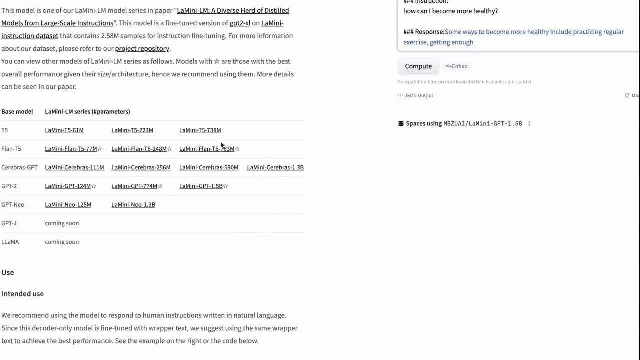 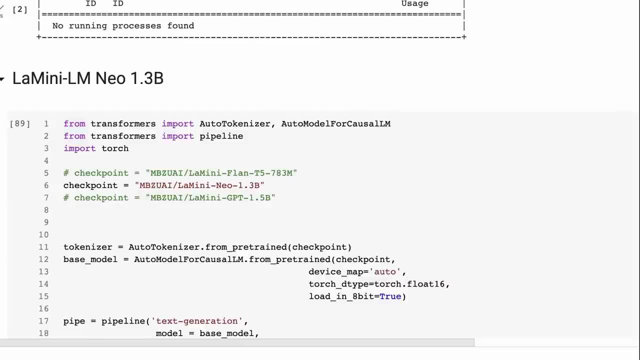 to pick three of these models to try out. I've gone for the Flan T5, the GPT-2 model, and the Neo model. So if we jump in and have a look at this, the first one I've got here is the Neo model. 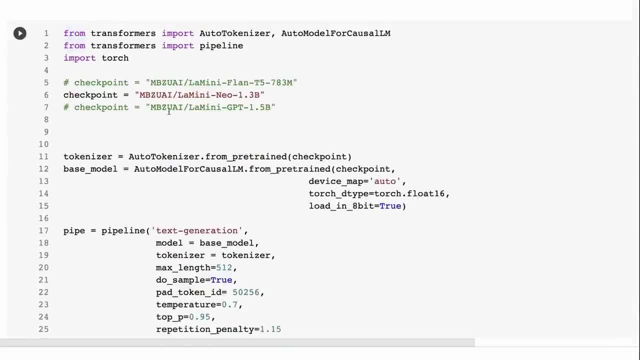 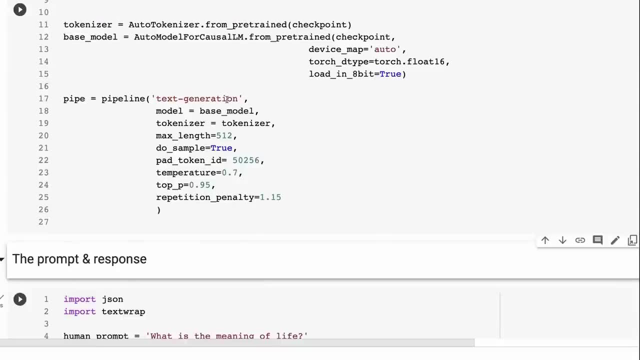 All right. And we've just got some simple code, for doing this. This is a decoder-only model. So we've got the causal language modeling, bringing it in, and we're just bringing a pipeline of text generation. 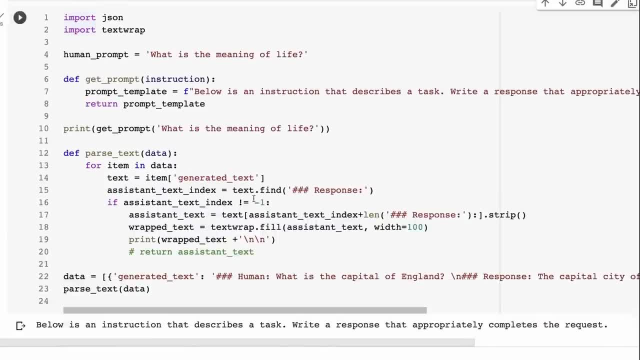 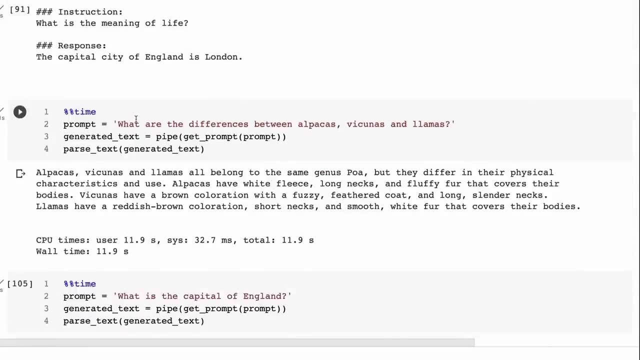 And I've just written some little code to sort of just tidy up the responses as it comes out of the model. And you can see that, okay, first off, we can ask it the general sort of questions that we've been asking it. What are the differences between alpacas, vicunas, and llamas? And you'll see that it's able to give us some information. Now, I'm not going to say that this is 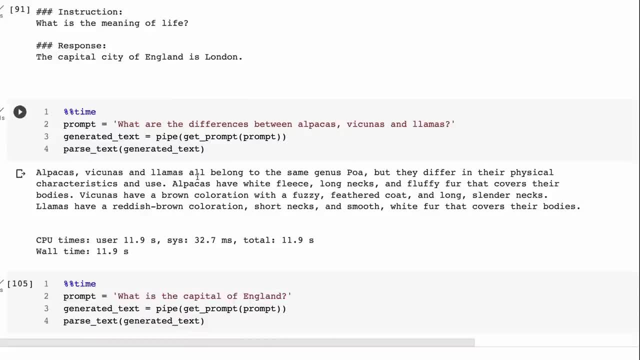 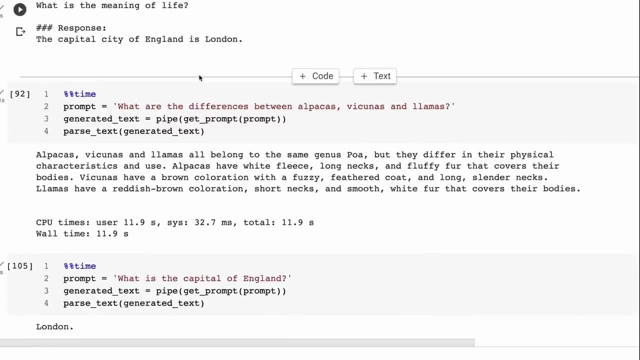 as good as the 7 billion models. Far from it, right? This is 1.3 billion parameters that we're looking at here. So the fact that it's even able to just stay on topic and stuff like that is 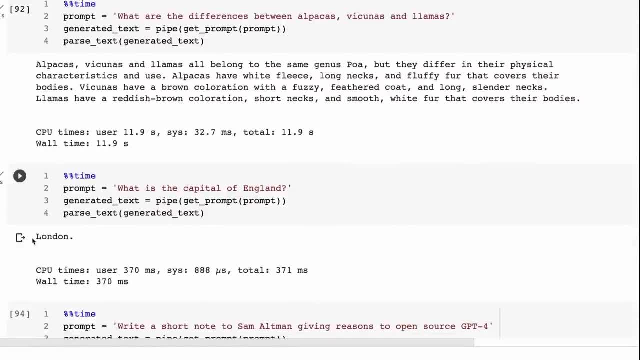 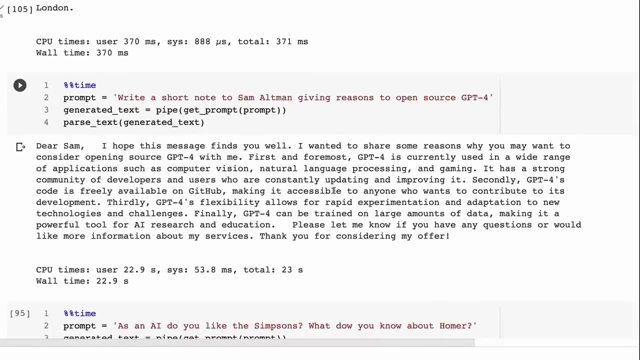 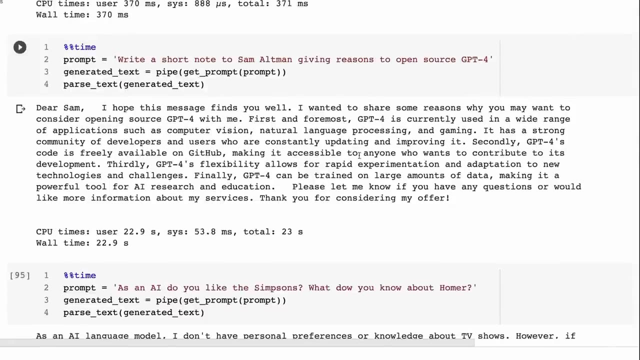 already a win for some of these. What is the capital of England? London. Write a short note to Sam Altman. So this one actually does a pretty decent shot at doing this. Much better than you'll see than some of the other models that we look at later on. It's definitely getting some facts and some information. So I'm going to go ahead and start. So I'm going to go ahead and start. 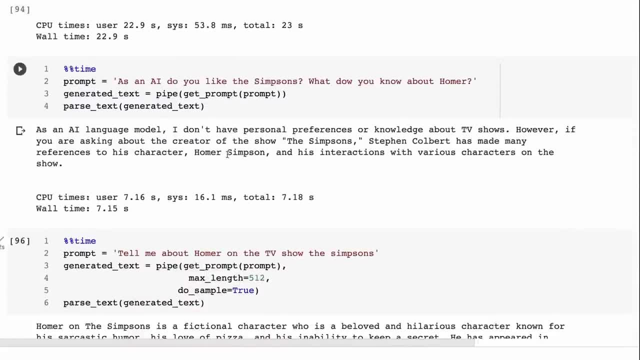 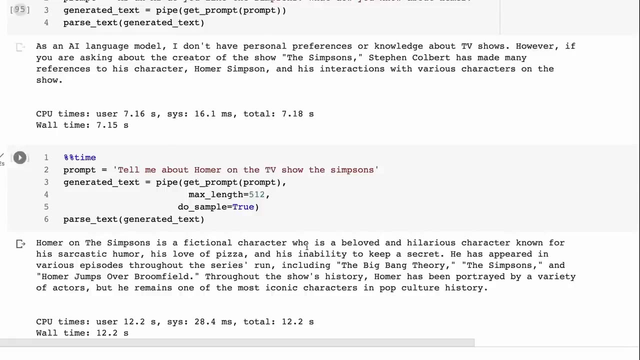 phrasing off though when we look at this of course because this has been trained on a distilled data set we're going to get the ai language model stuff in here unfortunately for some of these you'll see that it tends to hallucinate about some of these things i've done this one twice first time it didn't do very well second time it did a lot better so it is interesting that i probably don't see that as an ai language model as much as i see it in the packer or in the vacuna models etc my guess is probably just because of the diversity of the data set and the size of the data set 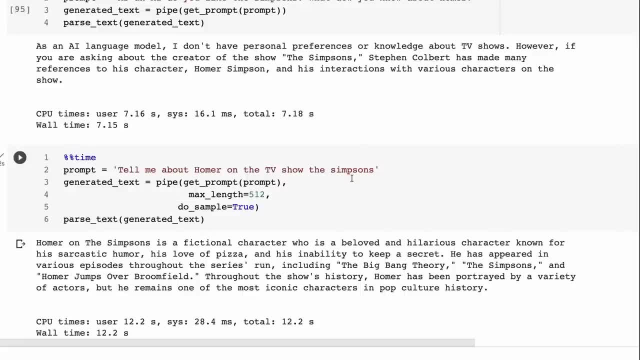 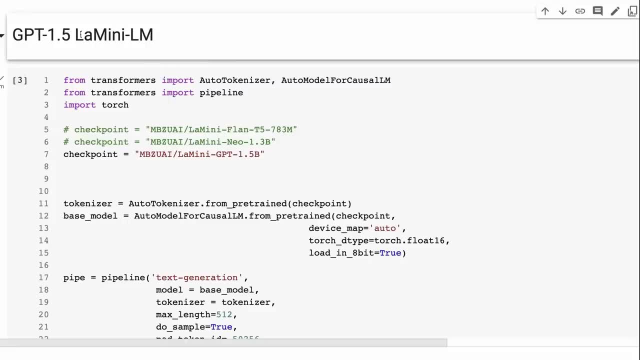 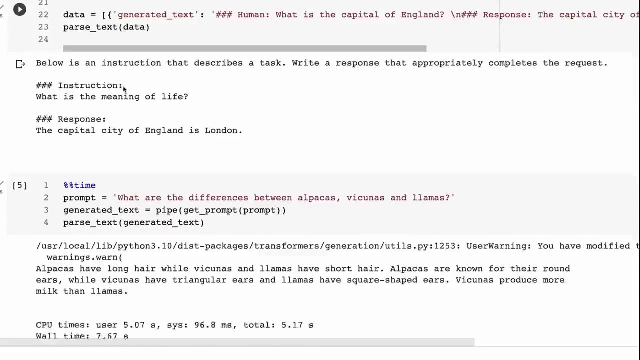 means that it doesn't see this as often as those other models see it let's jump into the next one just have a look at this one so this is the the gpt 1.5 billion lamini and so this is technically the gpt2 model that we've got in here same code etc for running this we can see that this is giving us responses again not kind of bad 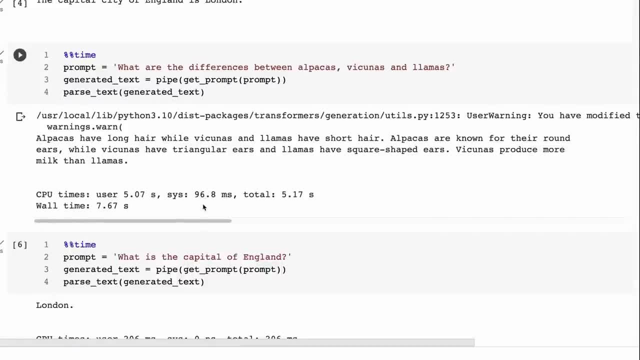 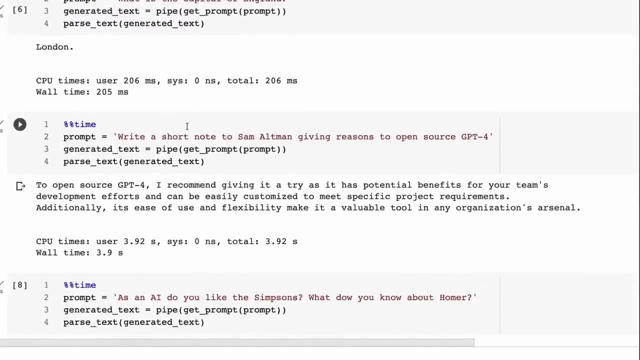 this is a little bit bigger than the neo one but i'm pretty sure it has to train on more tokens than gpt2 it's able to get some of these right it didn't do a great job at this write a short note to sam altman giving reasons to open source gpt4 a number of times when i ran this it just said noted or it said okay i will do that kind of thing here it's sort of saying to open source gpt4 i recommend giving it a try as it has potential benefits for your team's development 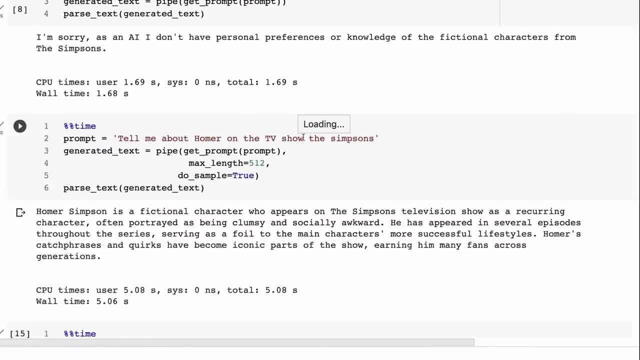 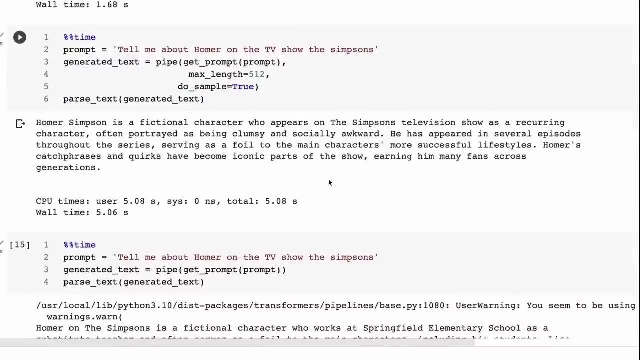 so i can see that the responses in here are pretty good we would not have expected this maybe from a gpt something like a dialogue gpt or something like that that was based on gpt2 in the past 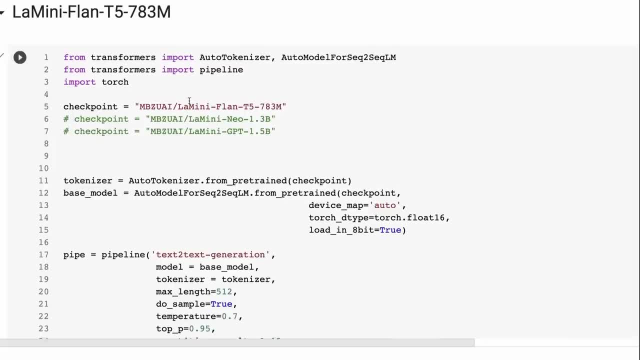 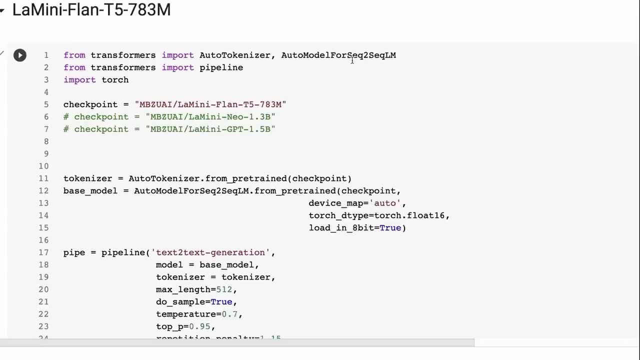 for these the final one that i look at is the the flan t5 one so this is actually half the size of the previous one now this is using this is a sequence to sequence model obviously it's an 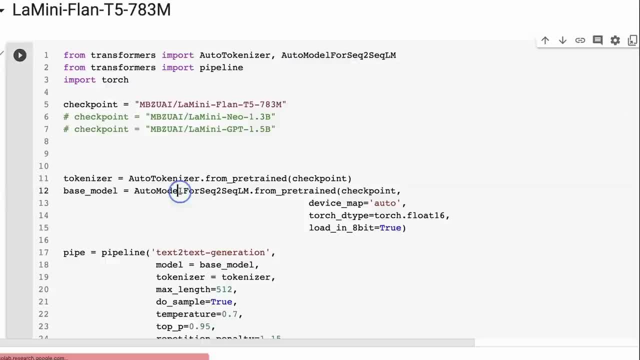 encoder decoder model for the t5 model so we need to use the auto model for sequence to sequence lms in there and we need to change the sequence to sequence lms in there and we need to change the 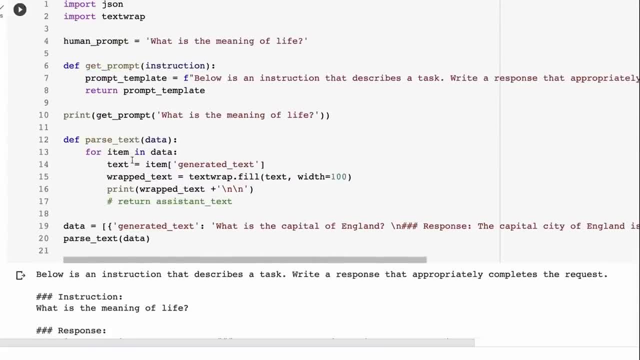 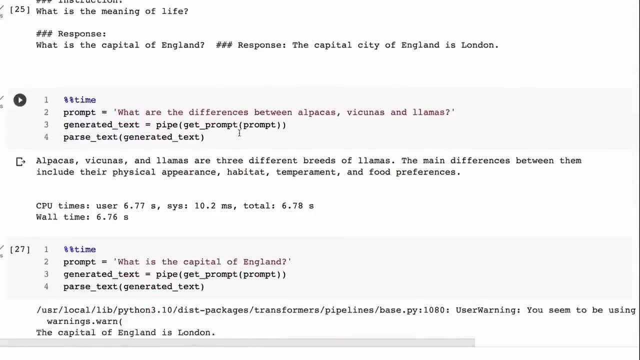 this to texture checks generation also i changed a little bit they seem to change the generation out from this a little bit so i've changed the filtering function there okay we can see when 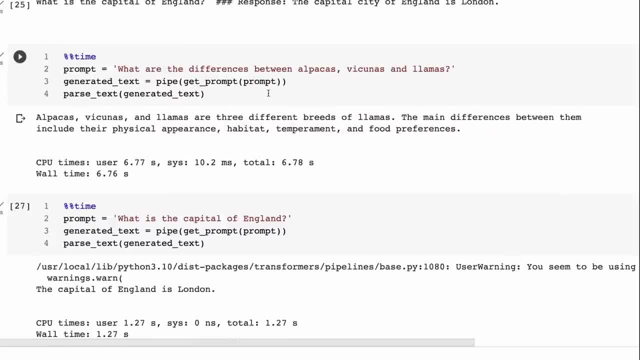 what are the differences between alpacas vicuna and llamas doesn't give us a great answer but it's definitely on topic here so you could imagine that we're doing a sort of general model here 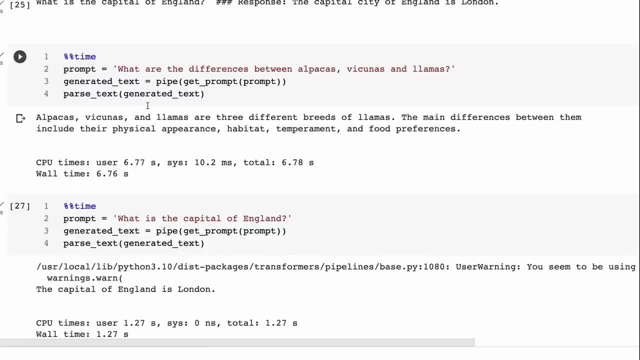 which is not how you would use these things these things are more for where you would basically hone in on one domain and train it up on a lot of data for that one particular domain 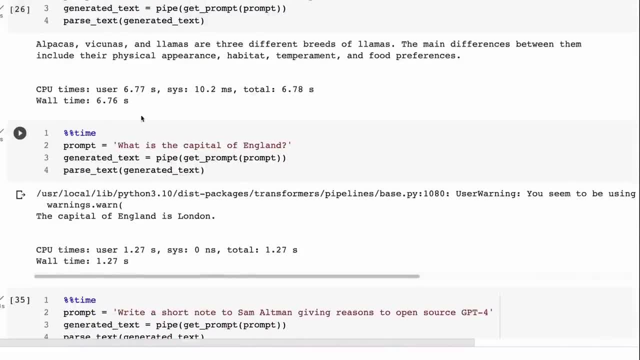 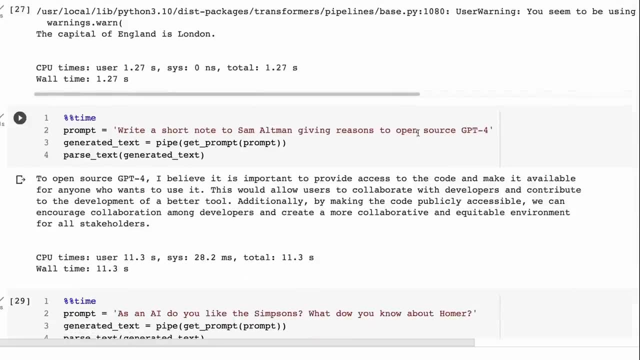 and get it going for that so that's something to think about what is the capital of england uh the capital of england is london write a short note to set only giving reasons to open source gpt4 and then it you know it's sort of done something around it we're definitely not getting 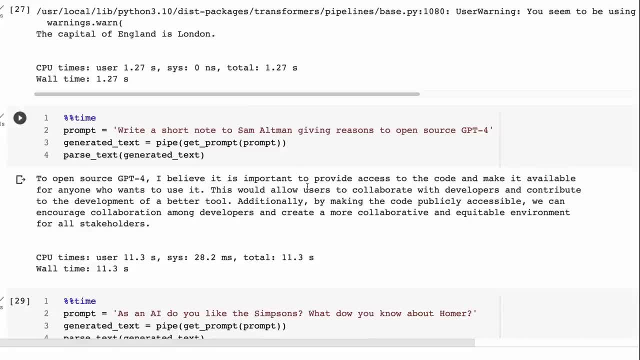 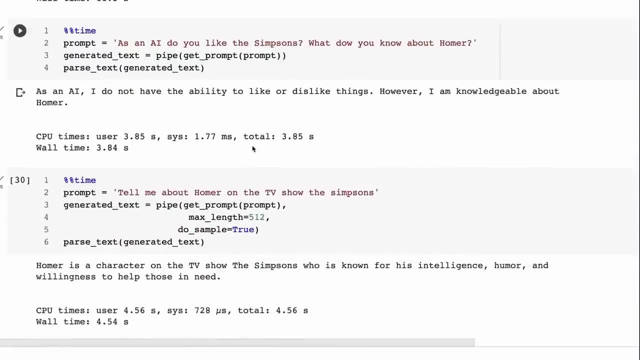 the you know in-depth responses that we get from vicuna 13 billion or something but we're talking about something that's 20 times smaller so it's not surprising in this case 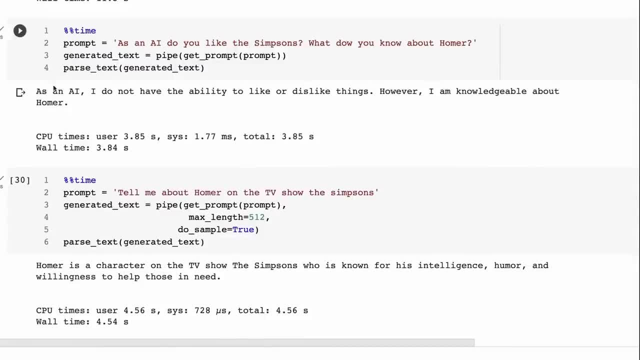 asking about homer so first off it basically uh does the whole as an ai i don't have the ability to like or dislike things however i'm knowledgeable about homer but it's quite sassy that it's not 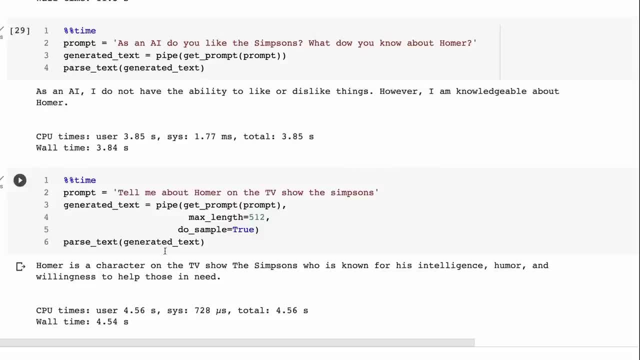 going to tell us what it knows about homer so ask it again and then here it gets oh yeah homer is a character on tv show simpsons who is known for his intelligence i'm not sure that is correct a humor 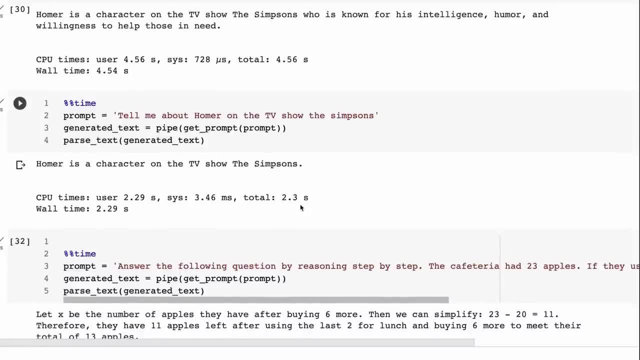 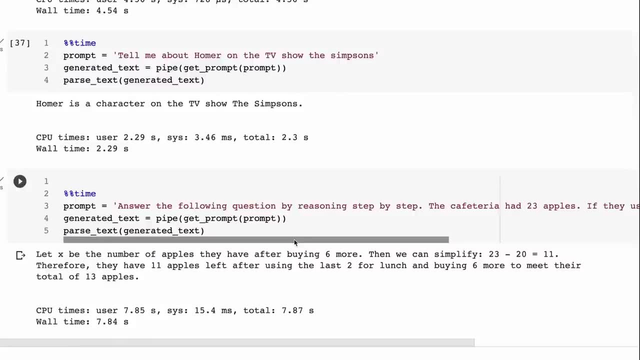 is to help those in need again not sure about that so you can see just different responses of that it gets out for those things none of them did well on the reasoning questions you know if we if 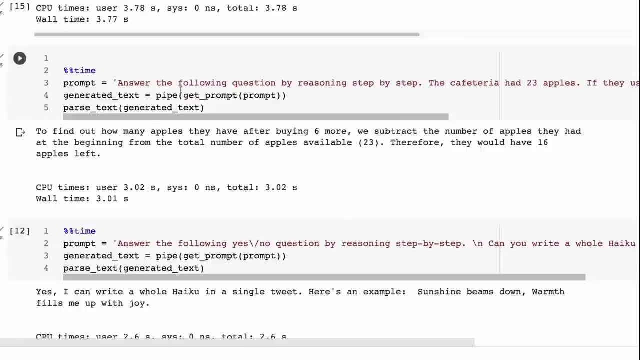 we sort of look at these i think it's the the reasoning one here it's basically saying that you would have 16 apples left not accurate although it does get the bit about a haiku 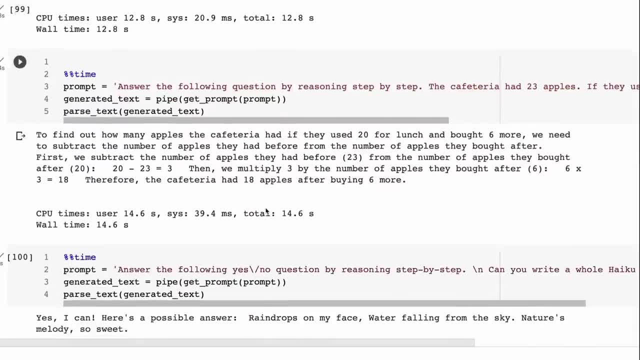 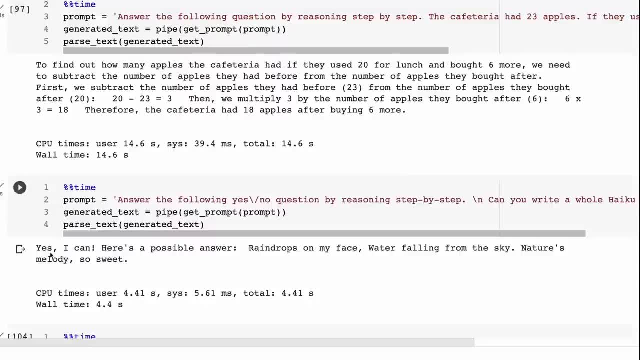 that yes that could be in a single tweet for the the neo model again it doesn't do a good job with the reasoning on the apples but it does an okay job with the haiku 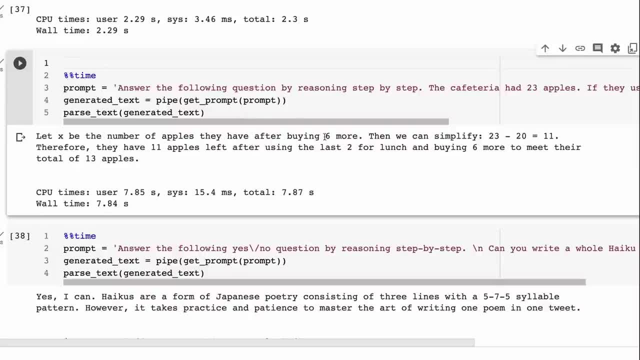 thing so this one also again not a great job at counting at working out those sorts of things but it does know a little bit about haikus in this case so anyway the goal here is not that 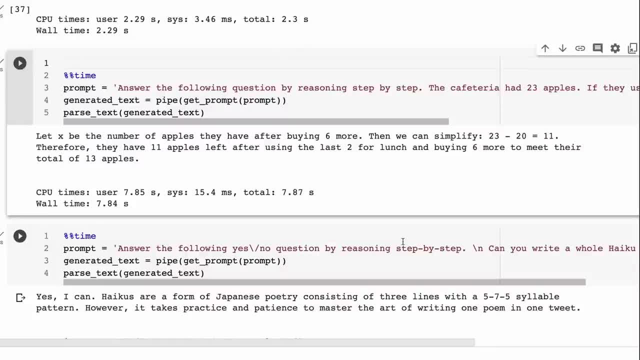 these are going to replace your general purpose vacuna or your koala model or something like that 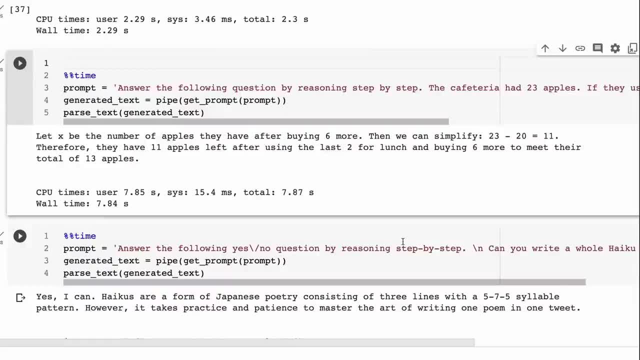 the goal here is that these are showing that if you train with a lot more data even a small model can get decent results with this kind of thing so you've got to think that as 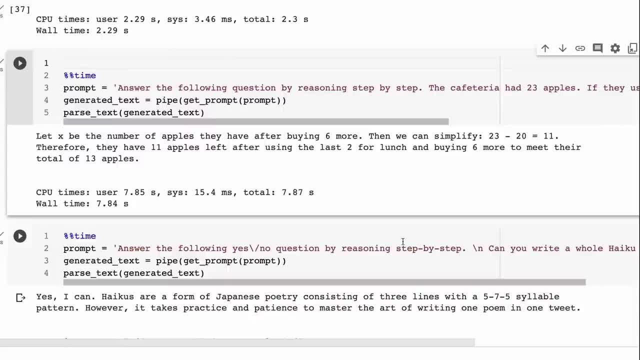 they bring out the 7 billion models and if they do them the 13 and 30 billion models on this 250 million data set it's going to be interesting to see 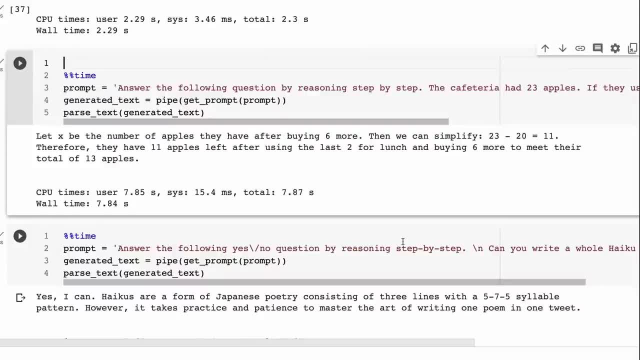 how they compare to the full vacuna models or the stable vacuna those sorts of models